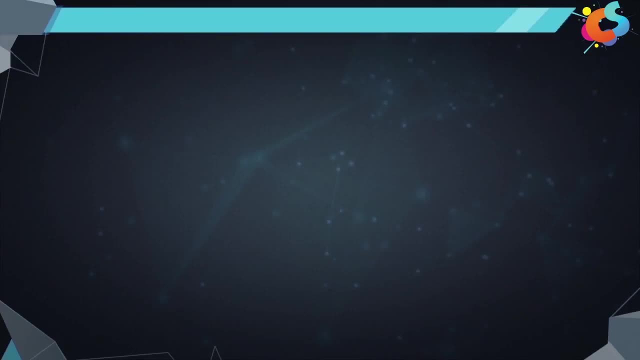 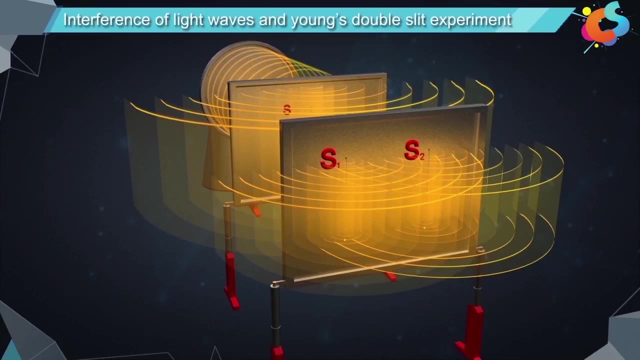 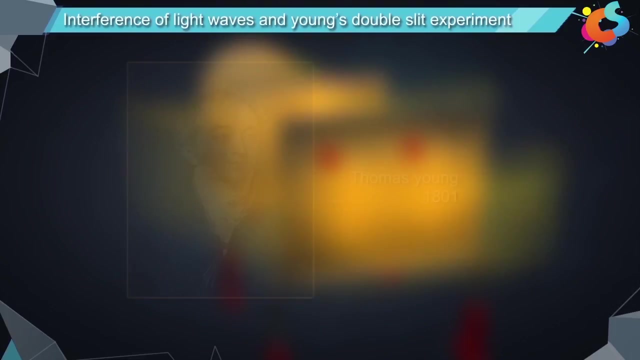 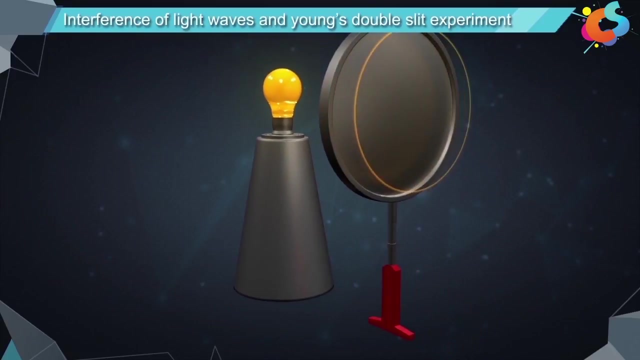 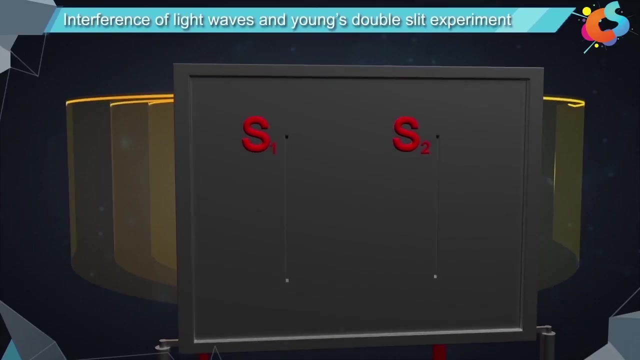 Interference of light waves and Young's double slit experiment. Now let us discuss about interference produced by light waves. This experiment was first carried out by British physicist called Thomas Young in the year 1801.. In Young's experiment, a monochromatic light from an illuminated slit S is allowed to fall on two symmetrically. 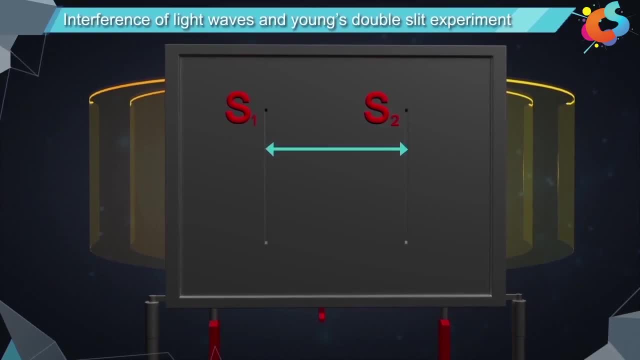 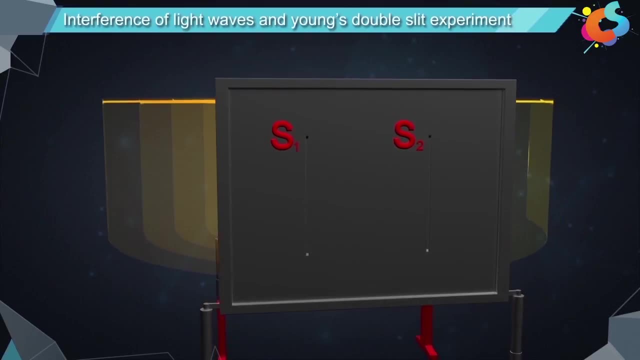 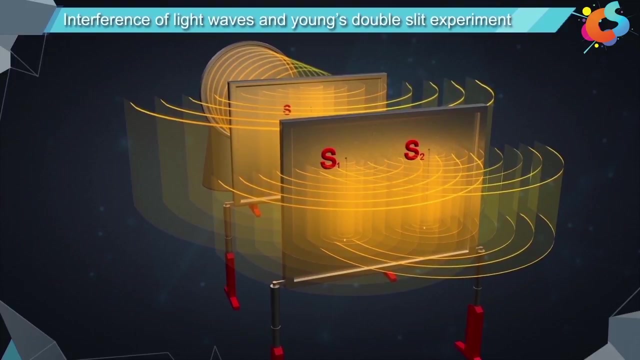 placed parallel slits S1 and S2 that are very close to each other and are at equal distance from the source S, The two slits start producing cylindrical wavefronts. Since the wavefronts produced by slits S1 and S2 are generated from a single original wavefront, they are 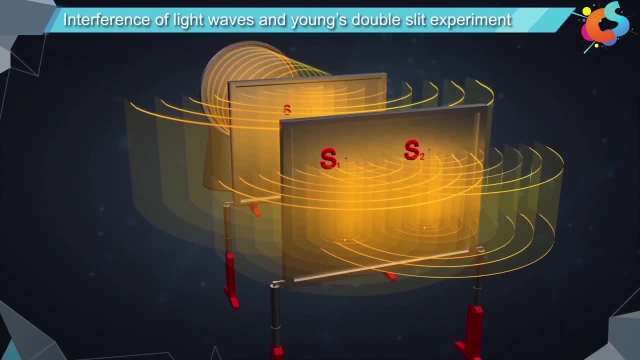 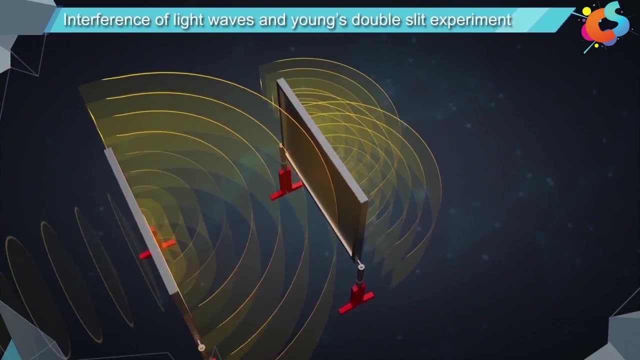 called coherent sources. The waves from slits S1 and S2 will have same wavelength, frequency and equal phase difference, Hence they can be called as coherent sources. The wavefronts emerging from slits S1 and S2 will interfere in space and produce a pattern. 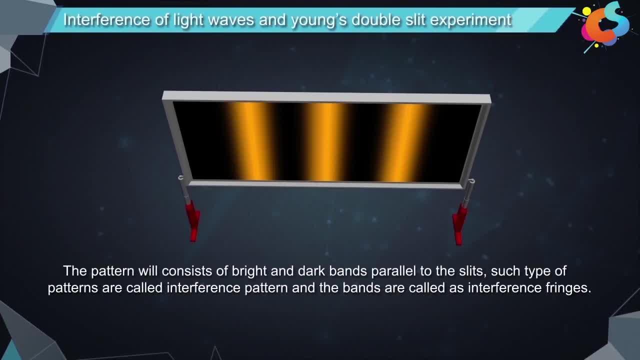 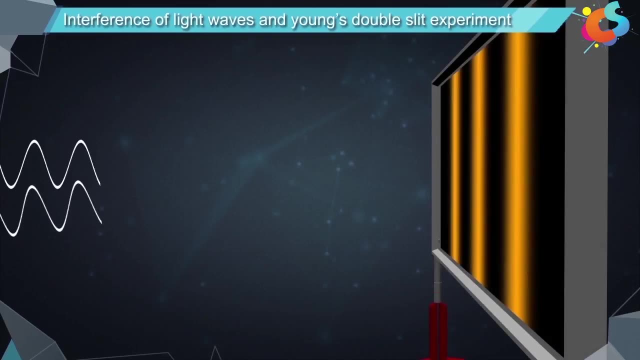 on the screen. The pattern will consist of bright and dark bands parallel to the slits S1 and S2.. Such type of patterns are called interference pattern and bands are called the interference fringes. Now, if two waves of light arriving simultaneously at a point, 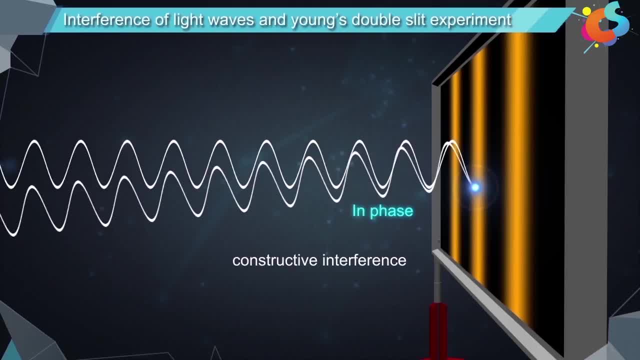 in space are in phase, constructive interference takes place. The intensity will be maximum at that point. Hence we get a bright fringe. Similarly, if two waves of light arriving simultaneously at a point are in phase, constructive interference takes place, Hence we get a. 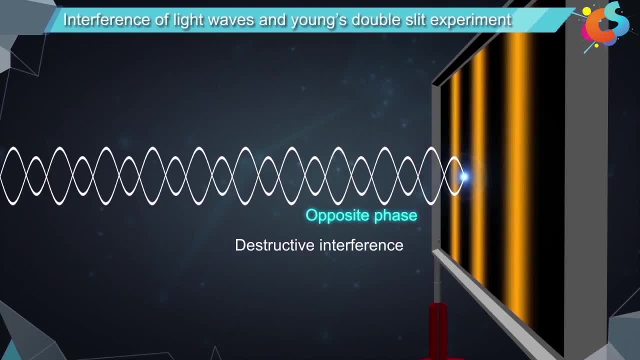 dark fringe In opposite phase or out of phase, destructive interference will take place. The intensity will be minimum or zero at that point. Hence we get a dark fringe. In this way, alternate bright and dark fringes are formed on the screen. 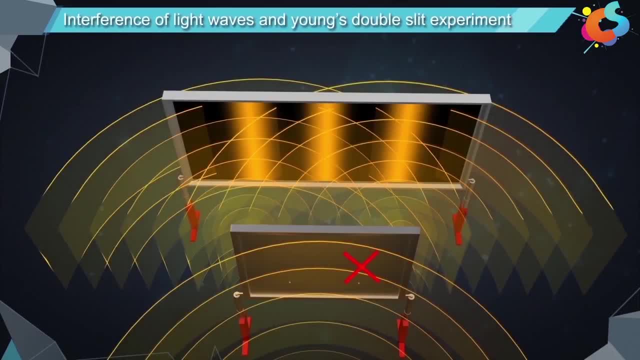 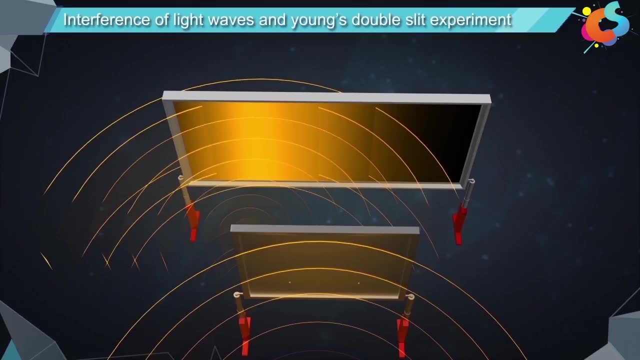 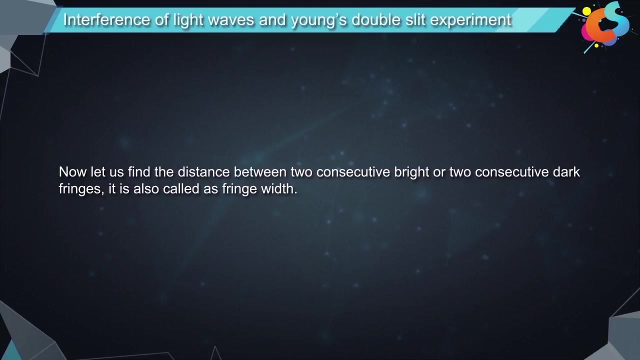 Now in this experiment, if we close one of the slits, the interference pattern disappears and we see only a plain light on the screen. This shows that two coherent sources are required to produce interference pattern. Now let us find the distance between two consecutive bright or two consecutive dark fringes. It 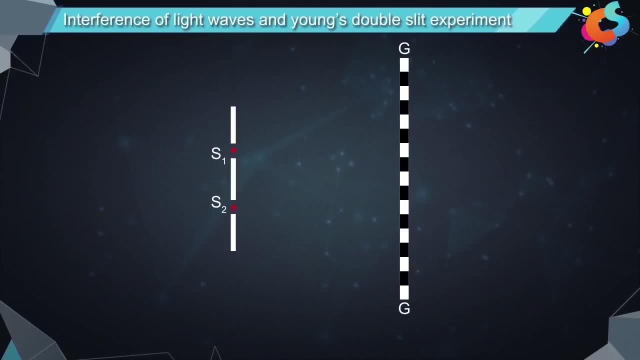 is also called as fringe width. Here let the distance between the two slits, S1 and S2, be small d, and the distance of the slits from the screen be capital D. The central bright fringe is formed at the point O, Since the point O is at equal distances from S1. 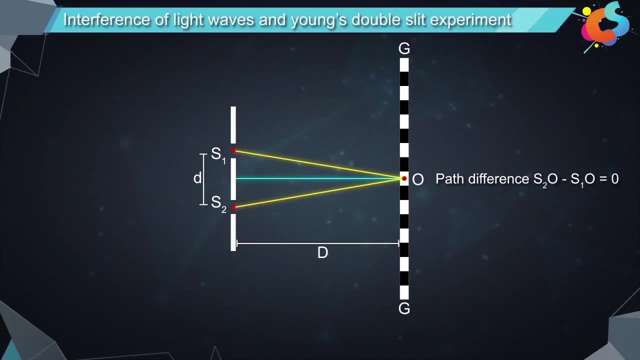 and S2, the path difference at this point S2O minus S1O is equal to zero. Now consider any arbitrary point P on the screen For a bright fringe. at point P, the path difference between the two waves reaching the point P. 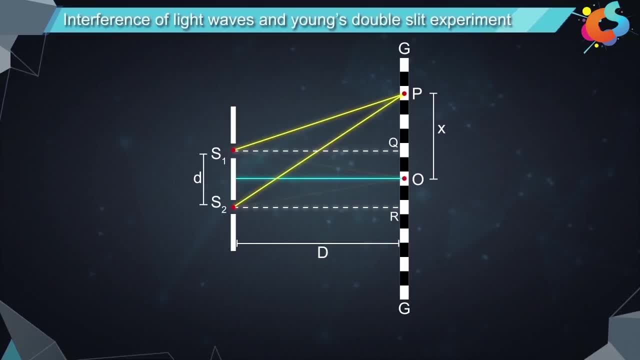 must be equal to S2O minus S1O. This is the path difference between the two waves reaching the point P. For a bright fringe at point P, the path difference between the two waves reaching the point P is equal to integral multiples of the wavelengths, that is n lambda, Therefore S2P minus S1P. 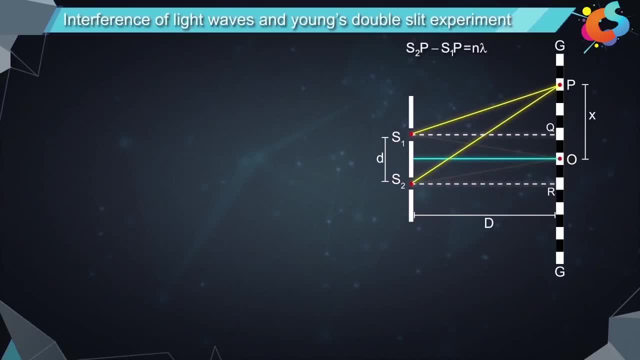 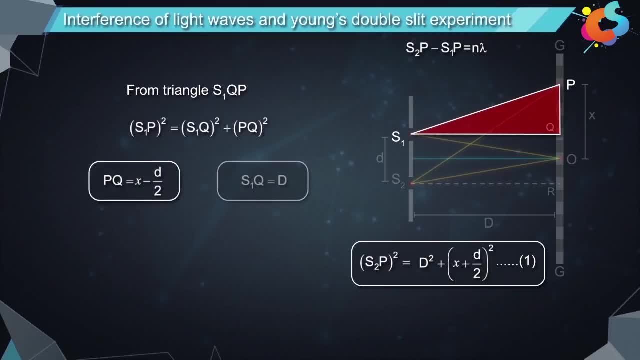 So S2P is equal to d and RP is equal to x plus r. So S2P is equal to d and RP is equal to x minus d by 2, and S1Q is equal to D. Substituting these values we get: S1P squared is equal to d squared plus x minus d by 2. 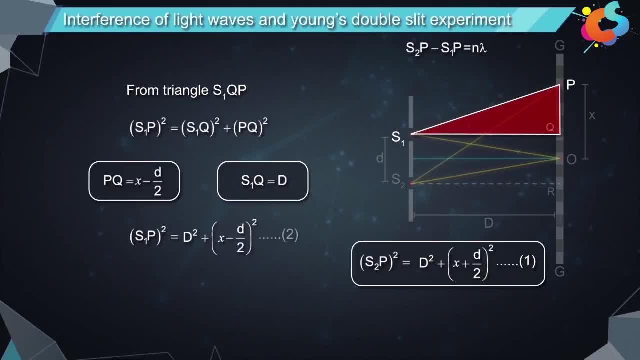 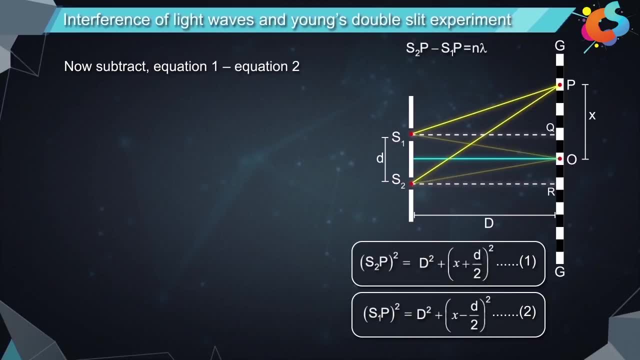 the whole square. Let�s call this a equation number 2.. Now, from equation one minus equation two, we get S2P squared minus S1P squared is equal to d squared plus x minus d by 2: the whole square. Let�s call this as equation number two. 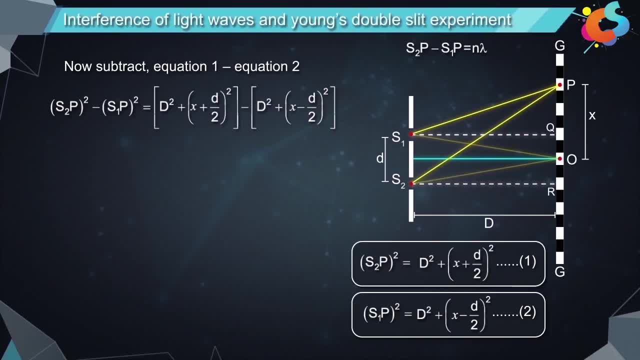 Next, from equation one minus equation two, we get xt verse 사람이 in x plus r, p2 is equal to d2 plus x plus d by 2 the whole. square minus d2 plus x minus d by 2 the whole. 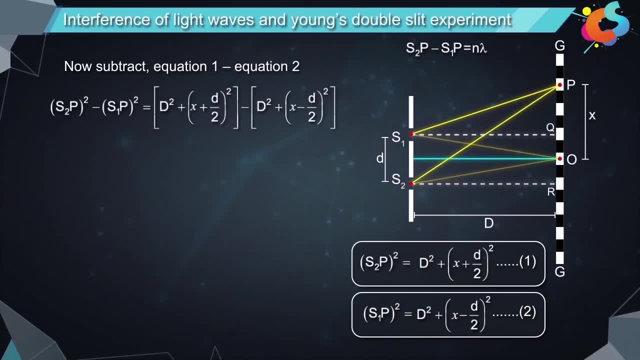 square. After simplifying this expression, we get s2 p2 minus s1 p2 is equal to 2xd. This expression can be written as s2p minus s1 p into s2. p plus s1 p is equal 2xd, or. 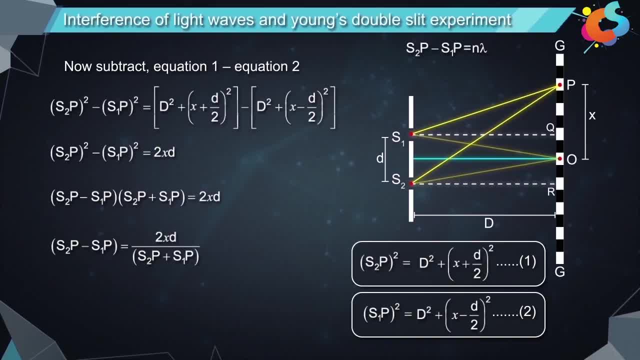 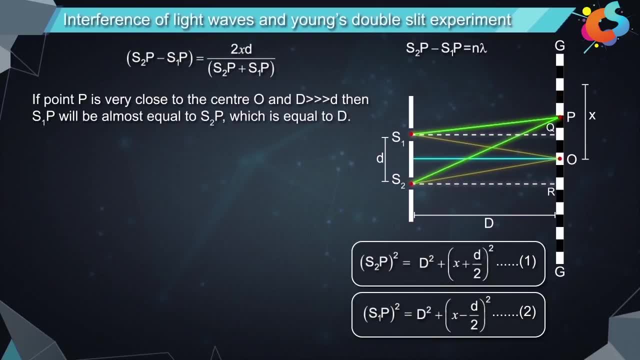 s2p minus s1 p is equal 2xd divided by s2p plus s1 p. If the point P is very close to the center O and capital D is far greater than small d, then s1p will be almost equal to. d. If the point P is very close to the center O and capital D is far greater than d, then s1p will be almost equal to 2xd. Then s1p will be almost equal to s1p plus s1p. 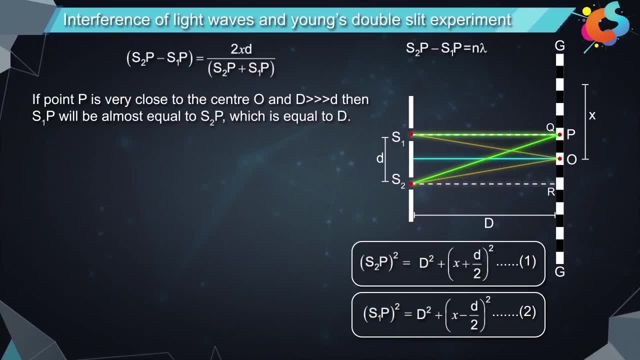 to S2P, which is equal to capital D. Therefore, S2P plus S1P is equal to 2D. Replacing S2P minus S1P by n lambda and S2P plus S1P by 2D, we get n lambda is equal to. 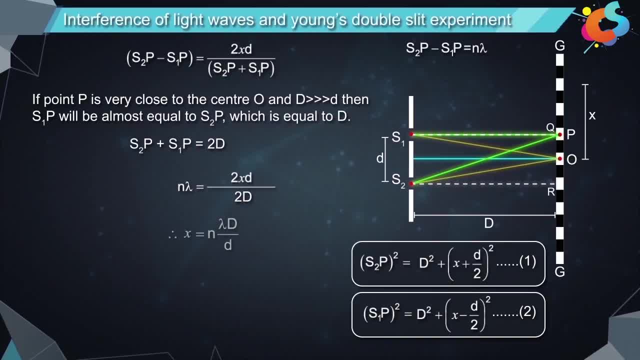 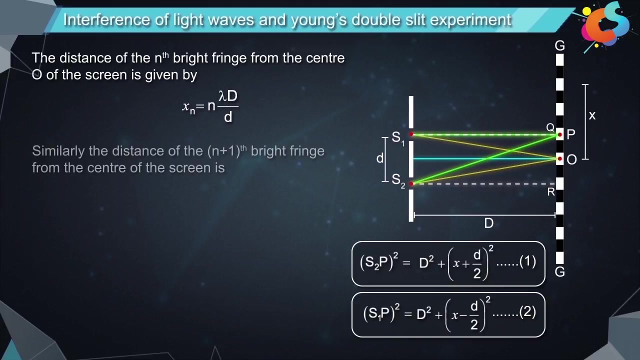 2XD divided by 2D. therefore, X is equal to n lambda D divided by D. The distance of nth right fringe from center O of the screen is given by Xn is equal to n lambda D by D. Similarly, the distance of n plus 1th bright fringe from the center of the screen is given: 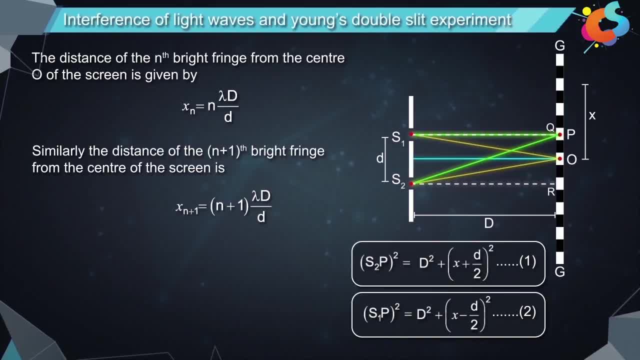 by xn plus 1 is equal to n plus 1 into lambda. d by d. The distance between any two consecutive bright fringes is called fringe width. It can be obtained by subtracting these two equations. Therefore, beta is equal to xn plus 1 minus xn, which is equal to n plus 1 into lambda. 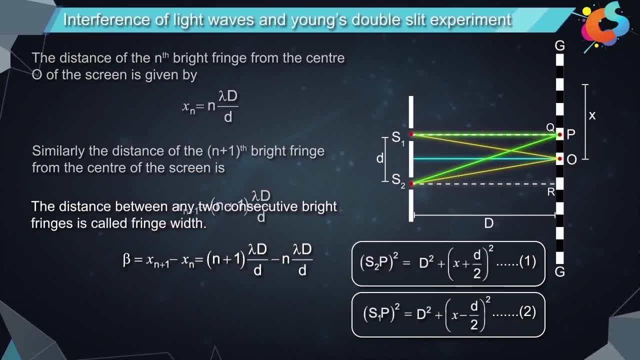 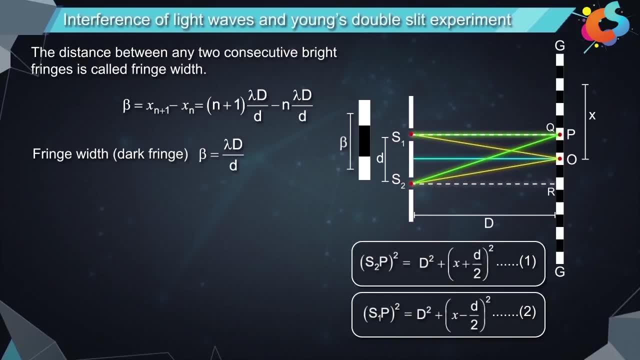 d by d minus n lambda d by d. On simplification, we get fringe width. beta is equal to lambda d divided by d. Similarly, if we calculate fringe width for dark fringes, we find that it is also equal to lambda d by d. 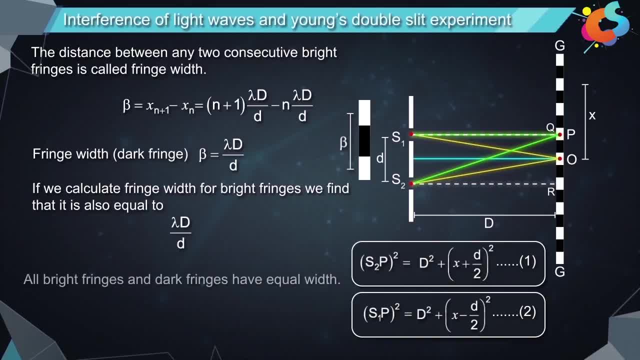 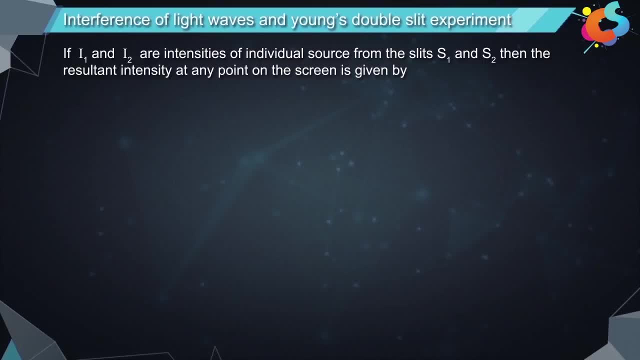 Therefore all bright fringes and dark fringes have equal width. If I1 and I2 are the intensities of individual sources from the slits S1 and S2, then the resultant intensity at any point on the screen is given by IR is equal to I1 plus I2 plus. 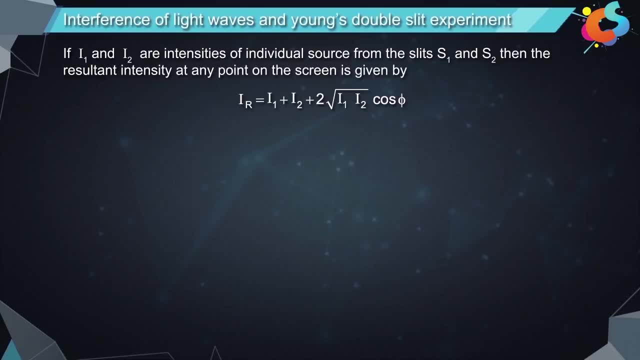 2 into root of I1, I2 into cos phi, where phi is the phase difference between the two interfering waves. If I1 is equal to I2, is equal to I0, then the resultant intensity is given by IR is equal to 4I0- into cos square phi by 2.. 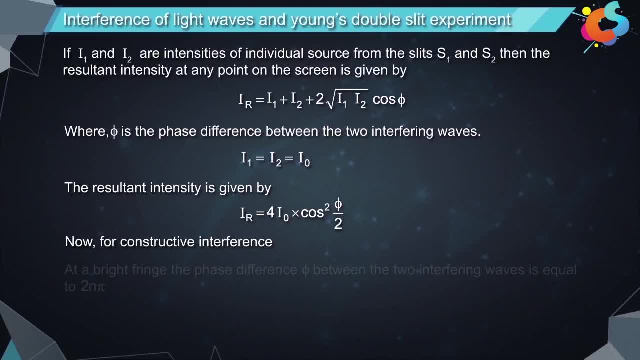 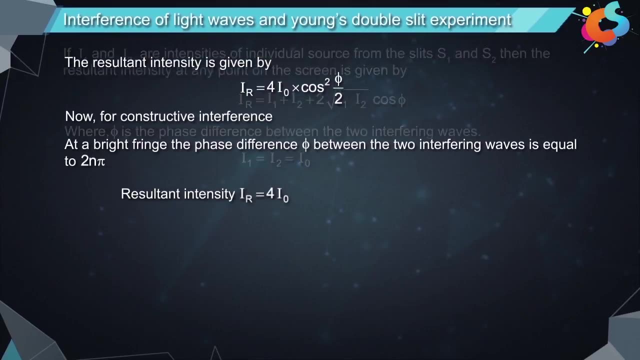 Now for constructive interference, that is, at a bright fringe, the phase difference phi between the two interfering waves is equal to 2N pi. Therefore resultant intensity IR becomes equal to 4I0.. Similarly, for destructive interference at a dark fringe, phase difference phi is given. 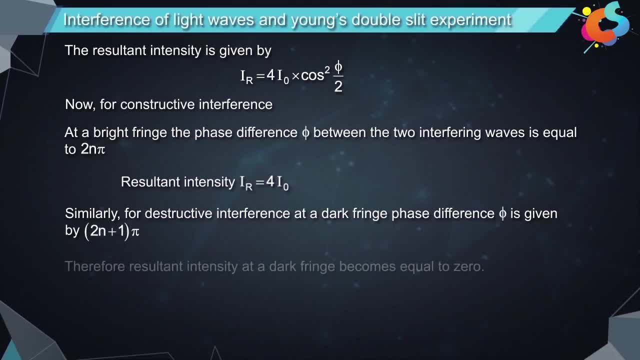 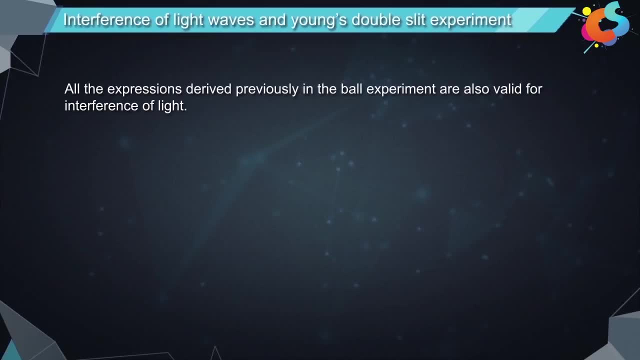 by 2N plus 1 into pi. Therefore, resultant intensity at a dark fringe becomes equal to 0.. Note that All the expressions derived previously are the same. The resultant intensity at a dark fringe is given by 2N plus 1 into pi. 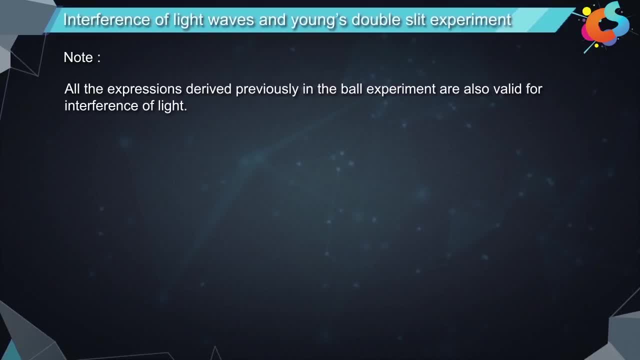 All the expressions derived previously in the ball experiment are also valid for interference of light. The intensity variation curve in Young's double slit experiment is like this: Note that All bright fringes are of equal intensity given by 4I0, and all dark fringes intensity. is found to be 0.. 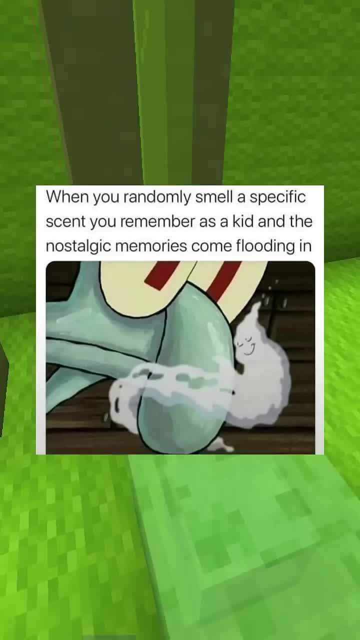 When you randomly smell a specific scent, you remember as a kid and the nostalgic memories come flooding in. Parents, when you laugh- once after you missed school for being sick, Grabbing coupons out of the dispenser for absolutely no reason, My mom Me telling my mom what I want to. 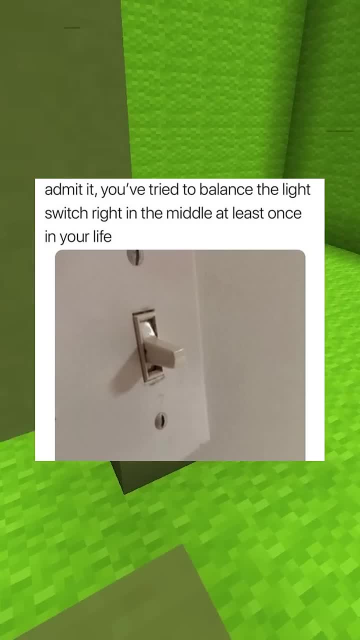 order from the restaurant. Admit it, you've tried to balance the light switch right in the middle at least once in your life. Before Snapchat and Instagram, this is where you showed off your outfit. When teachers teach you how to highlight, only highlight the important parts, Literally me. 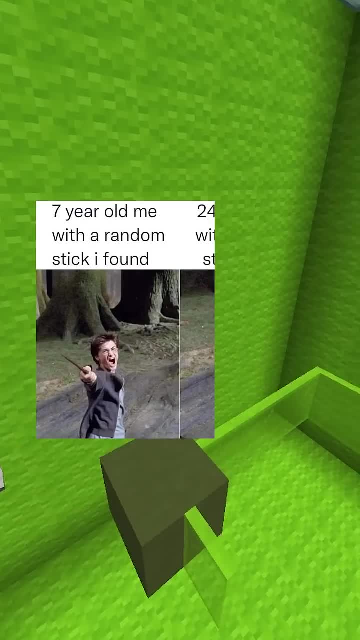 This is how it felt doing math homework with your dad- 7 year old me with a random stick. I found 24 year old me with a random stick. I found: Yeah, I'm a gamer. The game Did anyone else's mom make. 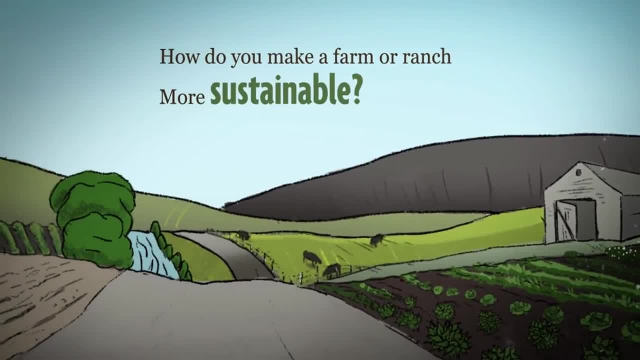 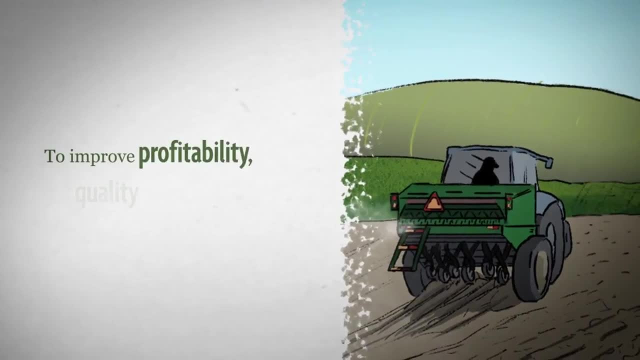 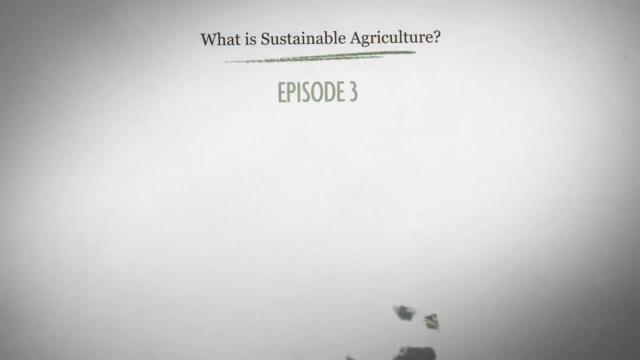 How do you make a farm or ranch more sustainable? There's no single answer, but there are some common practices used by producers across the country to improve profitability, quality of life and environmental stewardship. So in this episode, let's look at conservation. 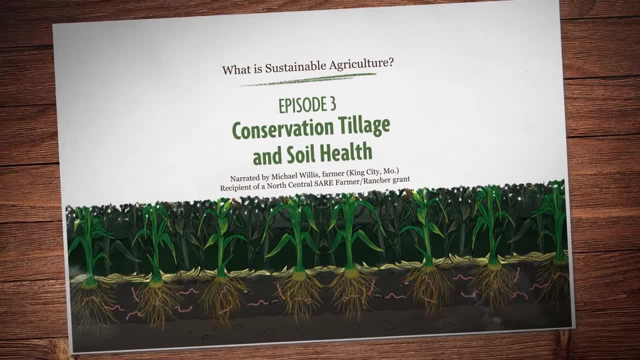 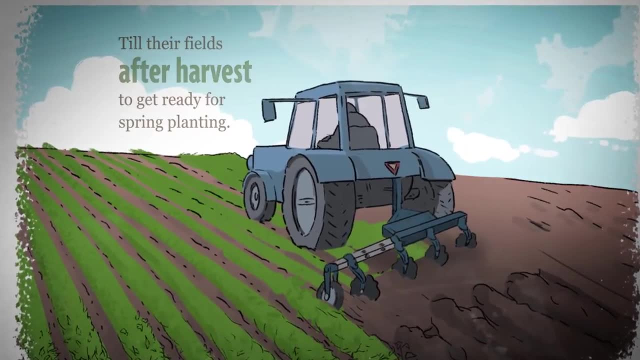 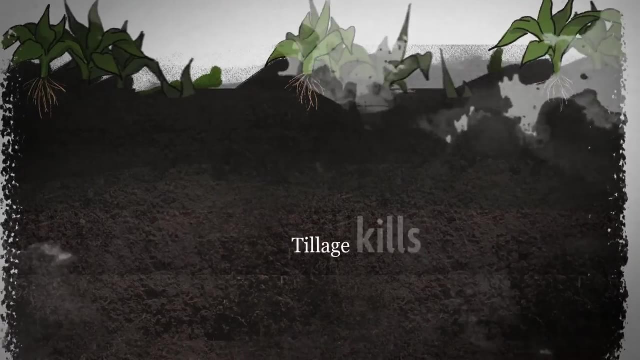 tillage and soil health. Now it used to be that every farmer in town would till their fields after harvest to get ready for spring planting. Now, besides burning a lot of time and fuel, we now know that tillage does a lot of harm to the soil. Tillage kills beneficial.